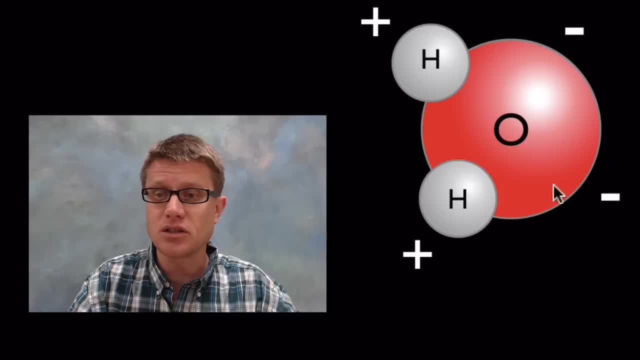 it's a polar covalent bond, And what that means is, since oxygen is pulling the electrons towards it, it's going to have partial negative charge on this side of the oxygen, And then the hydrogens are going to have a positive charge on the other side. And so if we were to add another molecule, 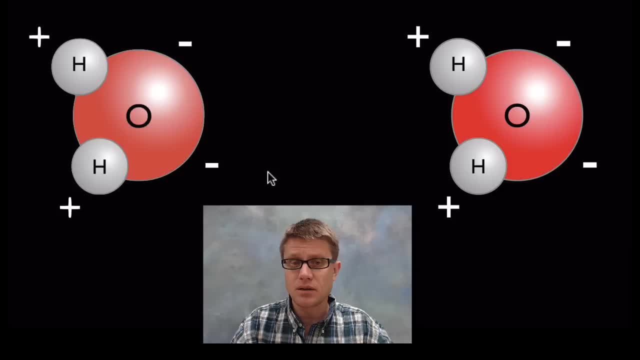 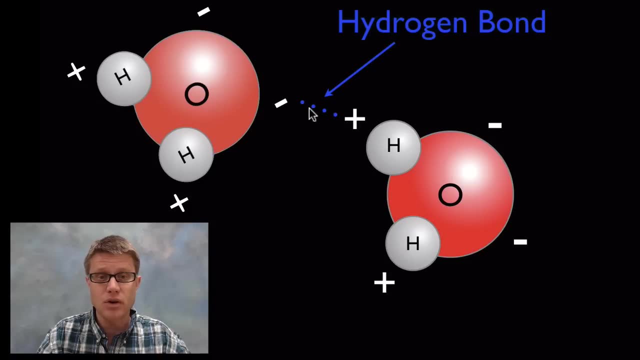 of water. these are not going to arrange this way, And in fact what we'll have is they'll be arranged like that, And so the hydrogen atom of one water molecule is going to be attracted to the oxygen of another, And that bond is called a hydrogen bond. A lot of students 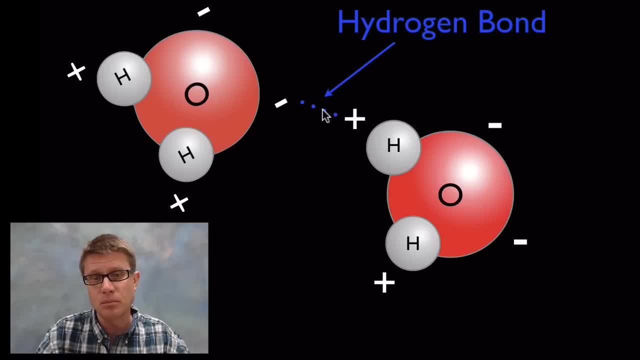 think that hydrogen bond is in here. No, That's covalent. But the hydrogen bond is going to be between the positive hydrogen, partially positive, and the negative oxygen. And that's why if we have one water molecule and the hydrogens are like positive and the oxygens, 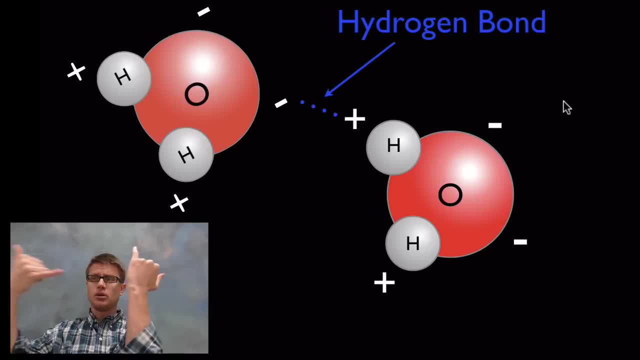 are negative and we have another one. they're going to line up like this And as I pull one water molecule, the other one is going to go along with it, And that's why we have cohesion and it explains a lot about water. But some weird thing happens with water Sometimes. 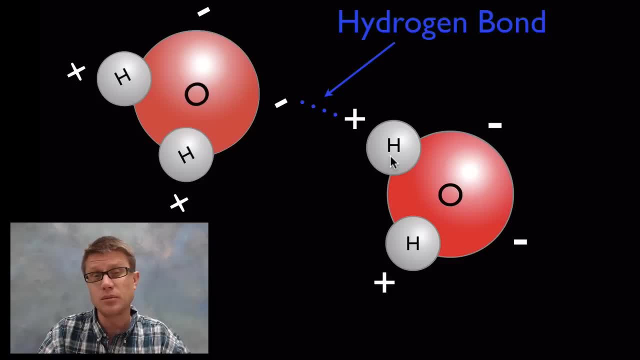 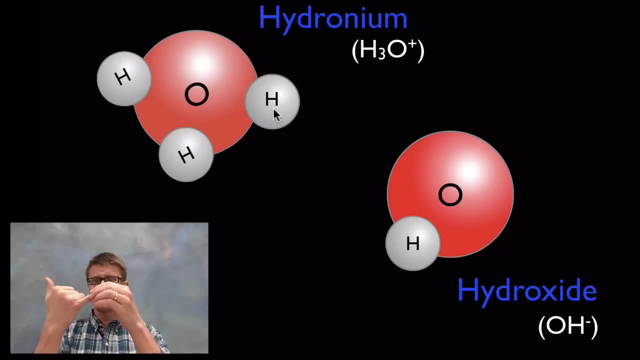 that attraction is so great that this hydrogen atom will actually become detached from the water and it will become attached onto this other water molecule. That would be like me pulling this pinky off and attaching it over onto this other water molecule, Leaving me just with this. And so what is that called? This is called hydronium. Hydronium is going. 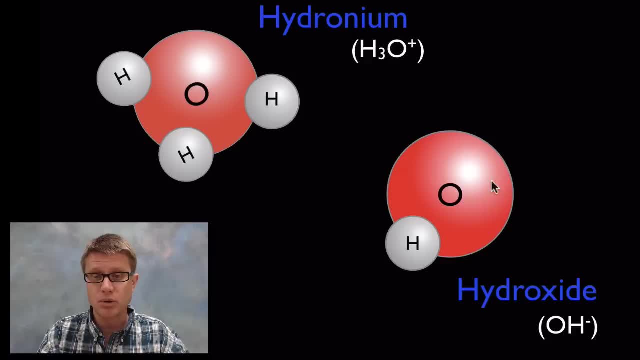 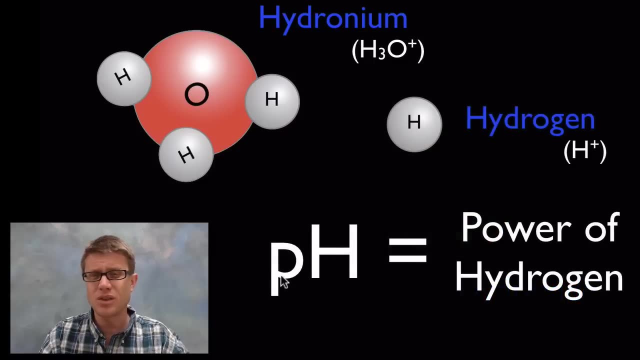 to be H3O, and it's going to have a positive charge. What are we left with over here? This is a hydroxide ion, And so what is pH? a measure of? Well, the P stands for hydrogen And the H stands, we think, for the power of hydrogen, In other words, the amount of hydrogen. But 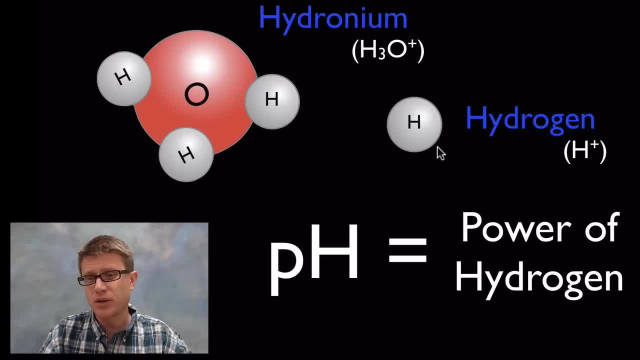 it could also be the amount of hydronium or the amount of just free hydrogen ion inside the water. And so if we look at the power of that, or almost the percentage of that, that's going to be what pH measures And in regular water, distilled water, the amount. 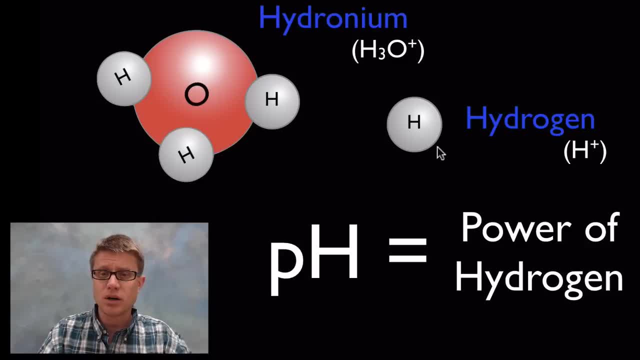 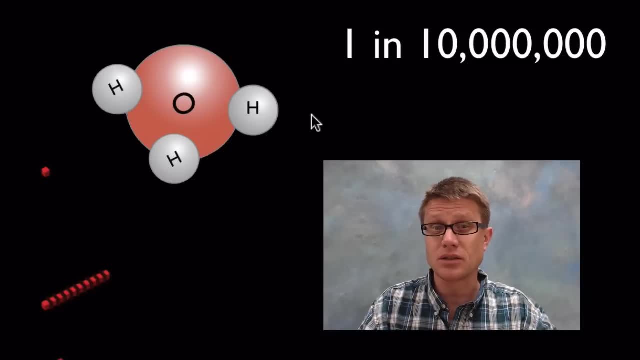 of this occurring is really really rare. In other words, it's a 1 in 10 million chance that we're going to have hydronium And that's going to be the amount of hydrogen that we're going to have, And this is really a molar concentration. So, to give you a sense of 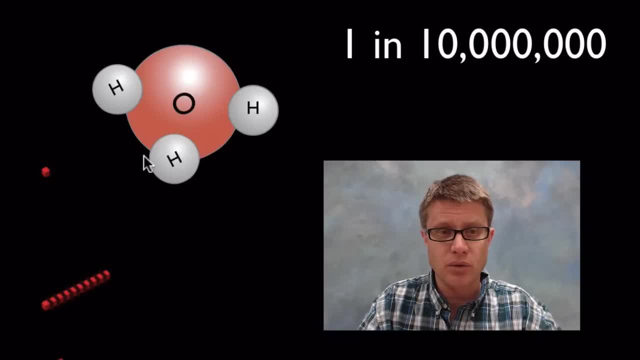 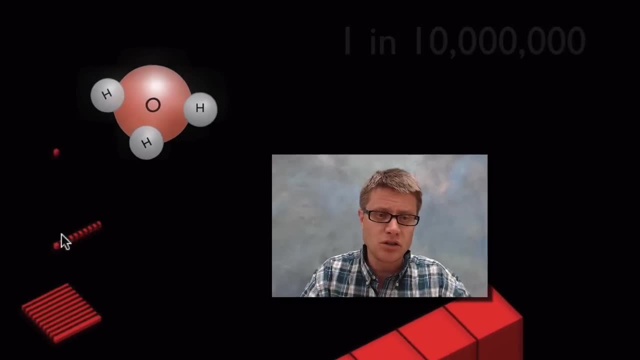 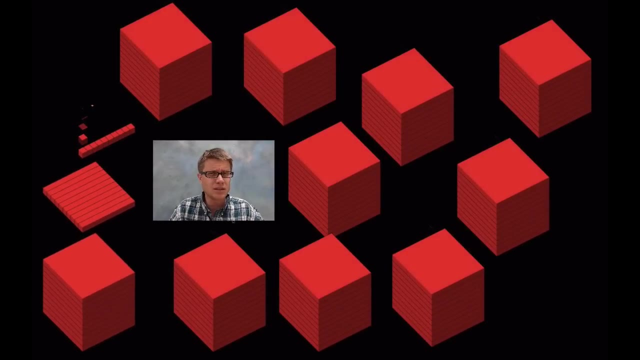 the scale. let's say, this hydronium ion right here is represented with this little cube, And so what I'm going to do is pull back And let's say this is 1 cube and 10 and 100 and 1000. And eventually what we get if we scale that, you really can't see that cube. 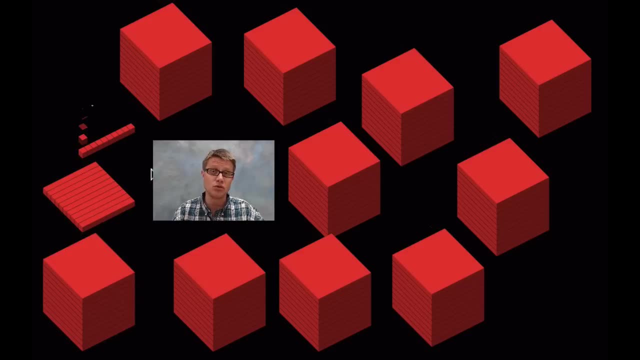 anymore, But this would represent 10 million cubes, And so the chances of that 1 hydronium forming are going to be really, really low. And so what we're going to do is we're going to take this 1 and 10 and 100 and 1000, and eventually what we get if we scale that. 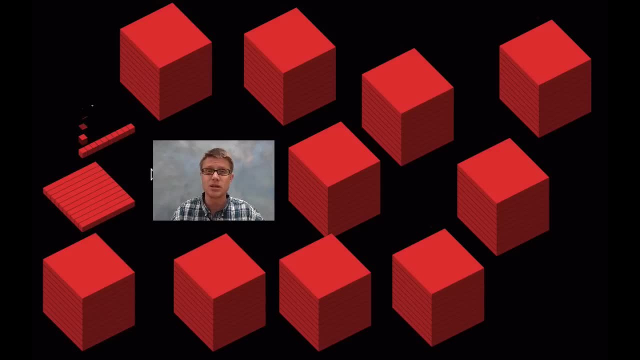 is. it's going to be low. But even though the probability of hydronium forming is low, it actually occurs in water and it has huge impacts on things that are found within that water itself, And so that 1 in 10 million. I want you to think about that for just a 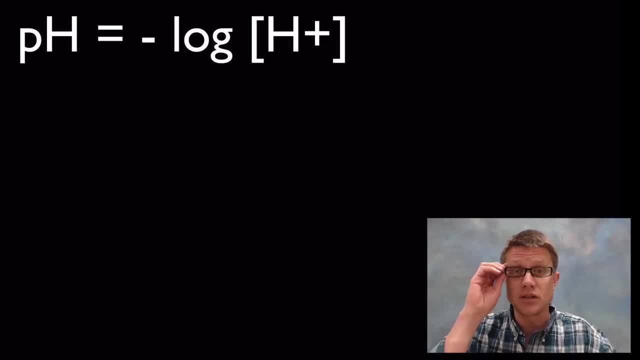 second, And let's kind of add a little bit of the equation of pH, And so some kids get scared by the equation. It's not that scary. So pH, or the power of hydrogen, is equal to the negative log of the hydrogen ion concentration, And so what we're going to do is we're going. 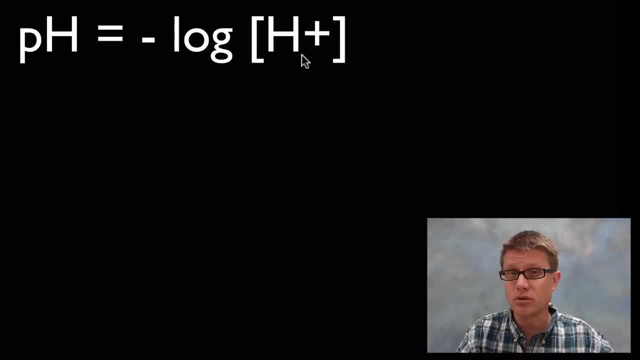 to take the hydrogen ion concentration, It's also the same as the hydronium That's at H3O+. Those are essentially the same thing. So it's the negative log of that, And so it's the negative log. think of this as 1 in 10 million, And this would actually be a molar. 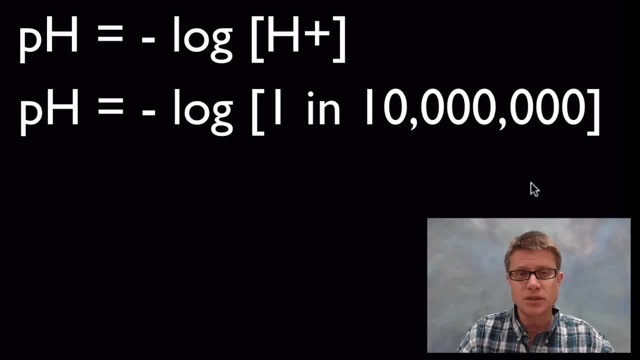 concentration. But we're keeping it conceptual right now, And so if we take the negative log of that, let's write 1 in 10 million in scientific notation, And so it's the negative log of 1 times 10 to the negative 7.. So this is going to be a really small number here. 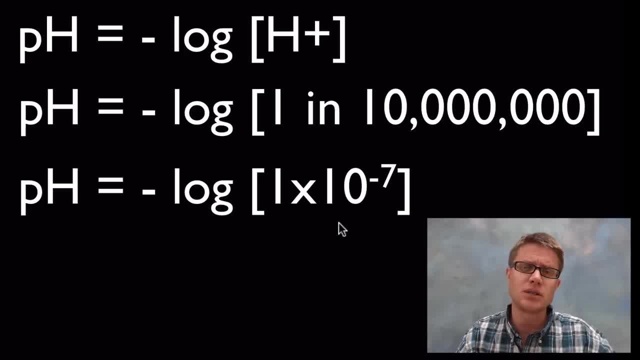 And this is where the math gets really easy. If you were to put this in your calculator. we take the negative log of 1 times 10 to the negative 7, what do we get? 7.. And so the pH is going to be 7.. And this gets us a number that we can actually deal with. And 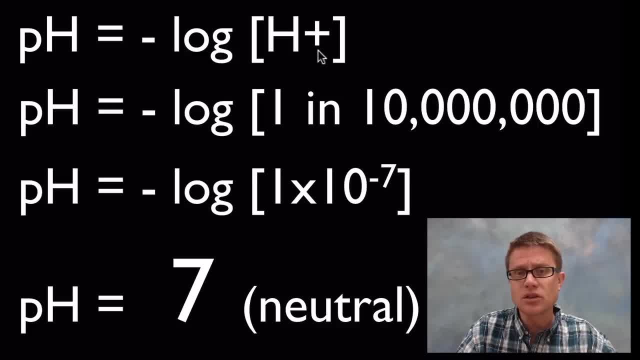 so what does it mean if the pH is 7?? It means that the concentration of this hydrogen ion is going to be really really small, And if we ever vary that, then we're going to be varying the pH. And so pH 7 is neutral. But if we ever have a 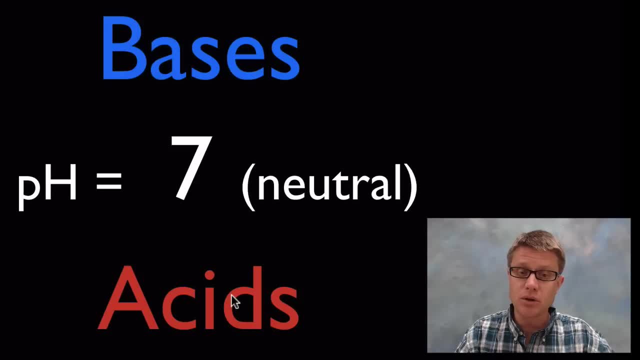 a value greater than 7, it's going to be a base, And if it's ever lower than that, then it's going to be an acid. And so let's start by dealing with the acids. What's an acid that almost everybody is familiar with? That's hydrochloric acid. You'd find that in your 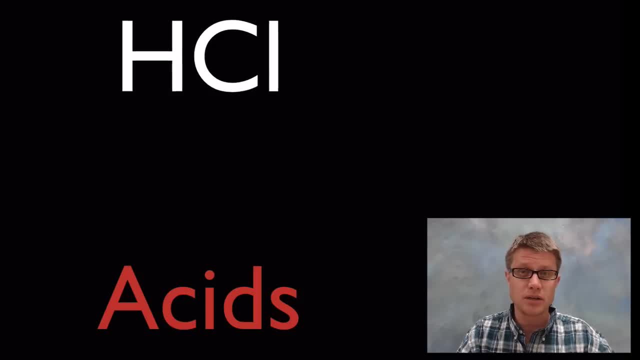 stomach. And so if we add hydrochloric acid to water, it's going to disassociate. It's going to break down into hydrogen ions and chloride ions, And so you can see here that we're increasing the amount of this H+, And so what is that going to do to that concentration? 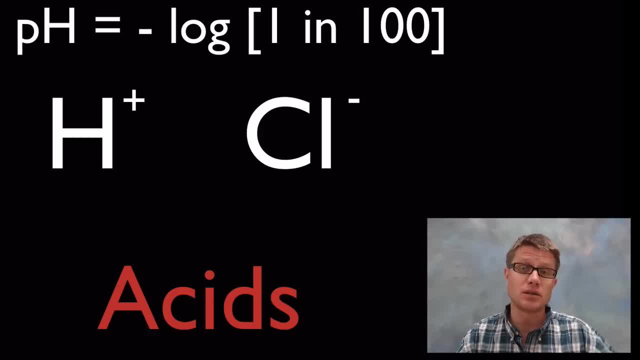 Now, instead of being 1 in 10 million, it might be as often or as common as 1 in 100. And so if we were to write that as scientific notation, it's the negative log of 1 times 10 to the negative 2.. So we would have to have pH of 2.. And so, depending on the concentration, 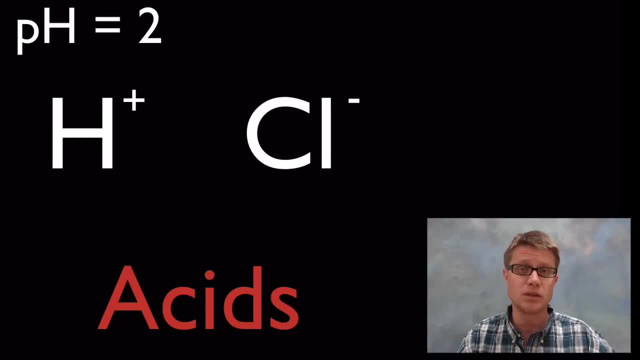 of hydrochloric acid. we could have a pH of 2 or 1 or 3.. It depends on how much hydrochloric acid is in there. Now let's look at a base, And so a base, for example, this would be sodium. 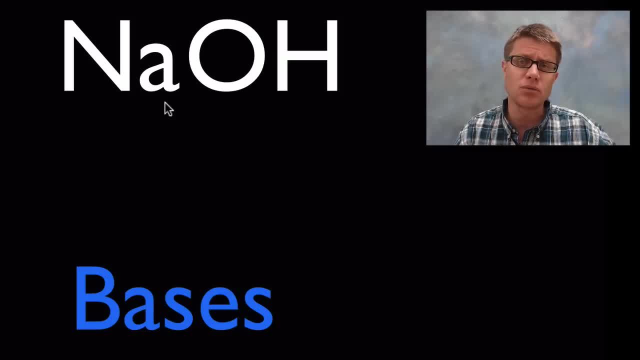 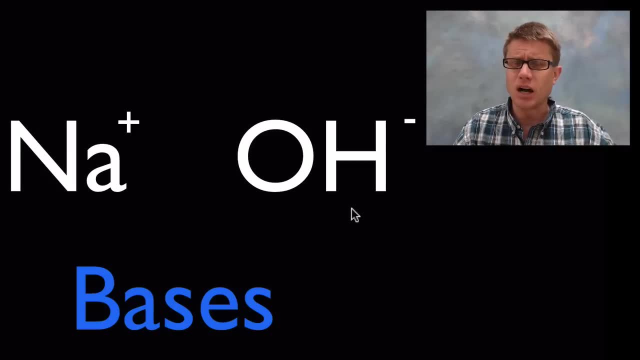 hydroxide or lye. Now what's going to happen to that? when we add it to water, It's going to break apart into sodium ions and hydroxide ions. Now that doesn't help us remember, because pH stands for the power of hydrogen ion. But what do you think is going to happen to that hydrogen? 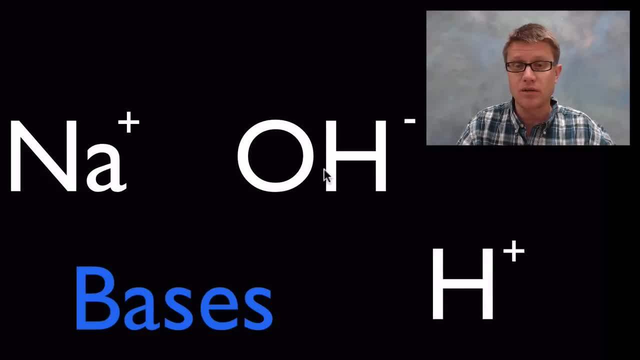 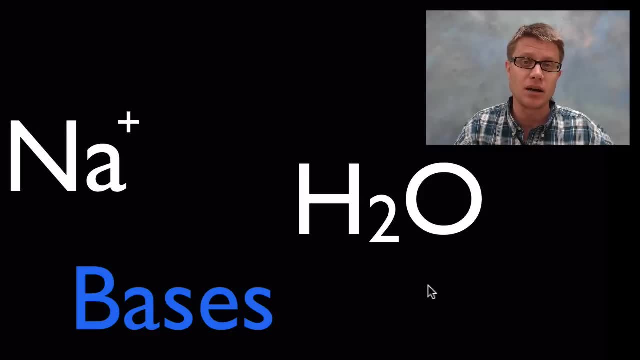 ion that happens to be in the water. Now we've got a hydrogen ion and we have a hydroxide ion And those are quickly going to combine to form water And as it does that, it's going to gobble up that hydrogen ion. What's that going to do to the amount of hydrogen ion? 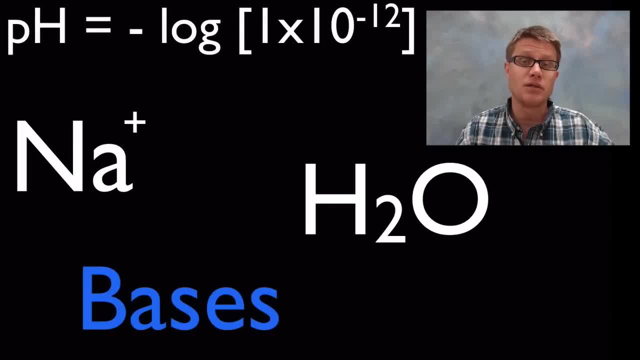 in the water, or hydronium ion for that matter. it's going to make it even more rare. And so now we have the pH equal to the negative log of 1 times 10, to the negative 12, for example. And so what's that going to be? That's going to give us a pH of 12.. And so what does pH? 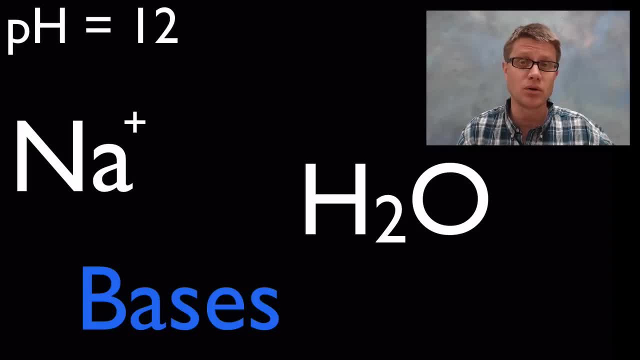 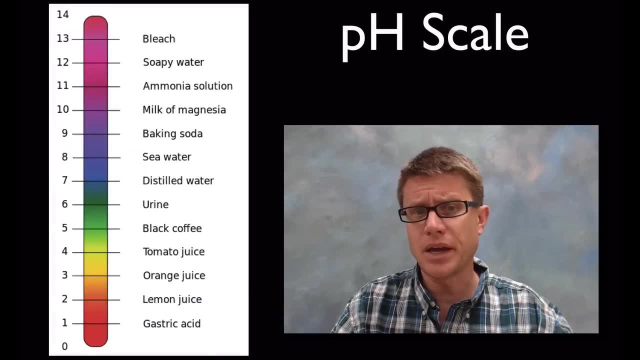 measure. It just measures the amount of hydrogen ions or hydronium ions, And bases and acids are going to have different amounts of that. We measure that using a pH scale, And so distilled water is going to have a pH of 7.. If we have anything higher than that, that's going to